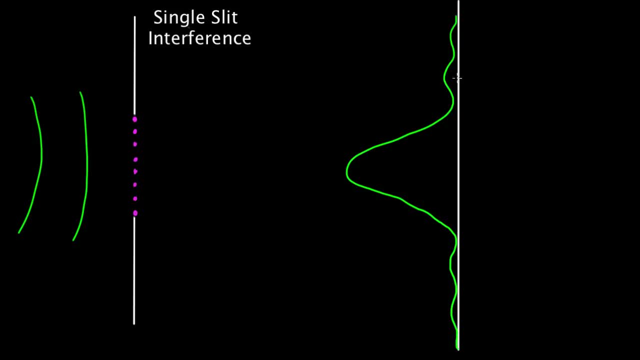 And I'd pick a constructive point right here. This is a bright spot, So this, if I had to give a guess for what point- would be totally constructive for all the waves, I'd say it's that point. So I'd take my topmost wave. I'd say it travels a certain distance to this bright spot. I'd take my wave in the middle: travels a certain distance to get here. I'd imagine my line straight down here to try to figure out the path length difference. 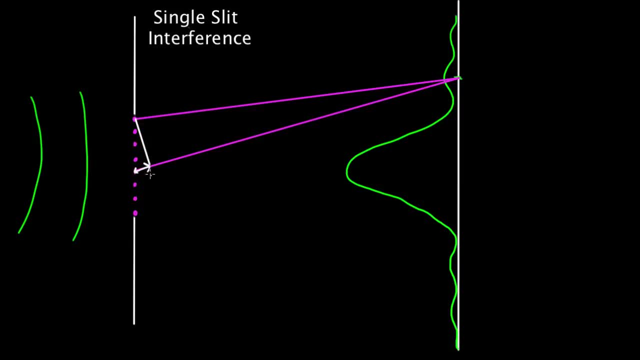 Now remember this: here is the path length difference. What should that be in order for these two purple waves? It's got to be an integer wavelength, So one wavelength, two wavelength. Since this is the first one from the center, we'll just say that's one wavelength. 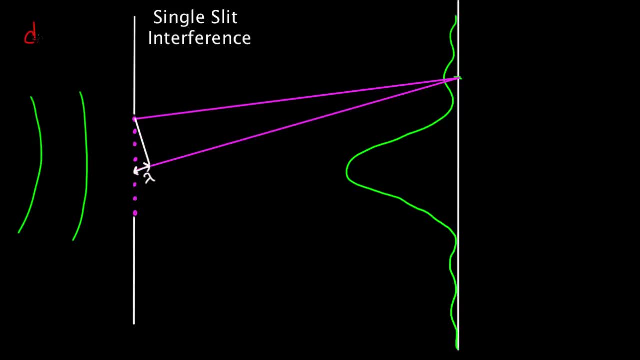 What's the relationship? We know that. Remember the relationship for the path length difference and the theta, the angle that it's at. Well, it's just d sine theta d is well, the whole width of the hole is a w. 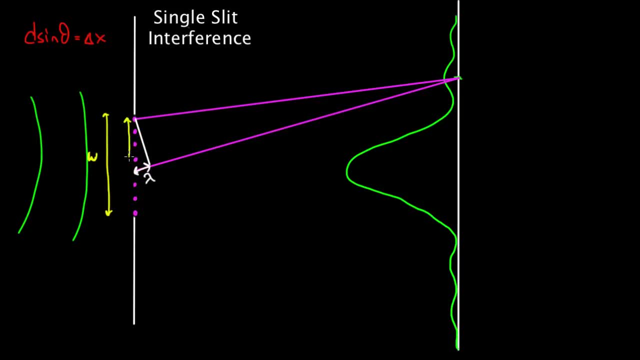 What width is this? This width between this source of light and this source would be w over 2.. And the relationship I'd get alright, d is w over 2 times sine of theta would equal. for this first point I'd say it's equal to lambda. 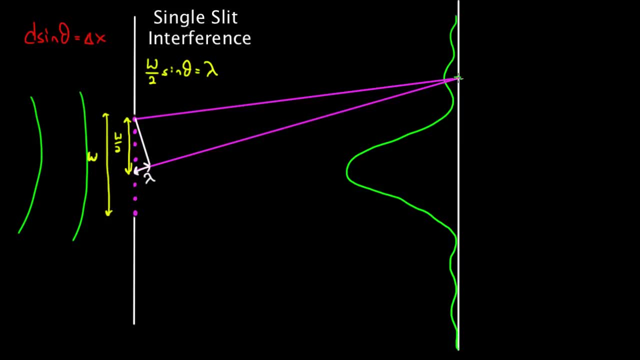 So let's just assume these two are interfering constructively at this point, And that would give me, w times sine theta equals 2 lambda. 2 lambda gives me a constructive point. Now I'm already confused. What w sine theta equals 2 lambda, constructive. 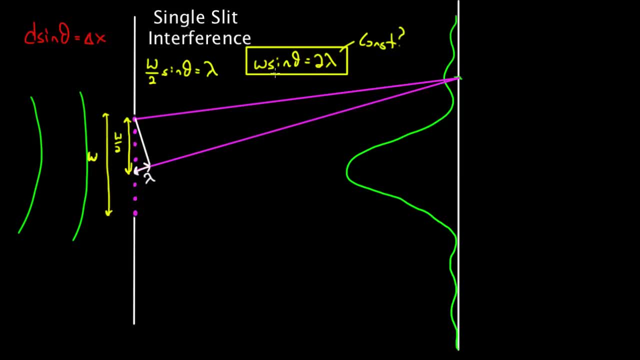 We already proved this is a destructive point. Remember our relationship for the destructive points that we derived was: w sine theta equals m lambda, as long as m is not 0, but 1,, 2,, 3,, 4,, 5.. 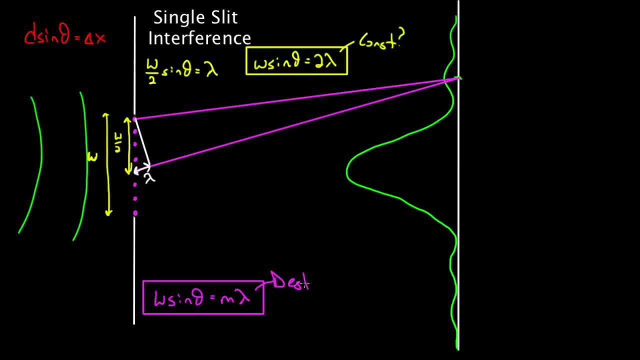 These are giving destructive for any m equals 1, 2.. It could even be negative. if you want to consider down here any integer, It looks like we've just proved these are constructive. How are these constructive? Well, they're not really. 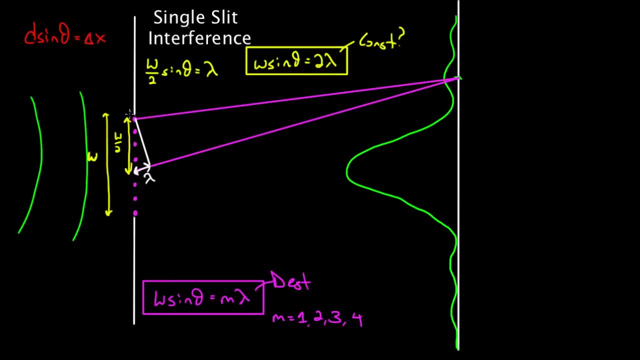 They kind of are, but watch what happens. Just here we go. So if I follow this argument through, the thing that fails- our previous argument is fine. The argument that fails is this current one with constructive points, Because, yes, these two are constructive there, but watch. 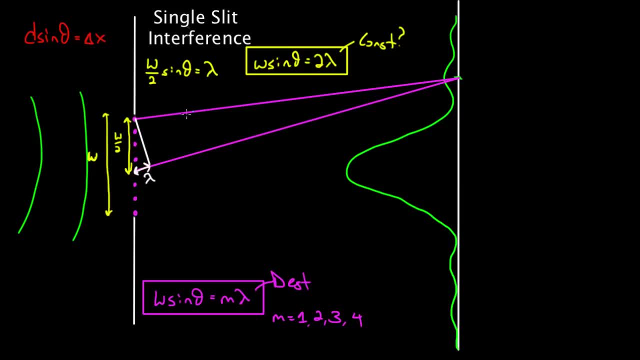 This point here. Remember the game we played. We said: if these two are constructive, then the rest of them should all be constructive. Is that so? Well, let's go down one. Let's go down one. I imagine these two waves getting here. 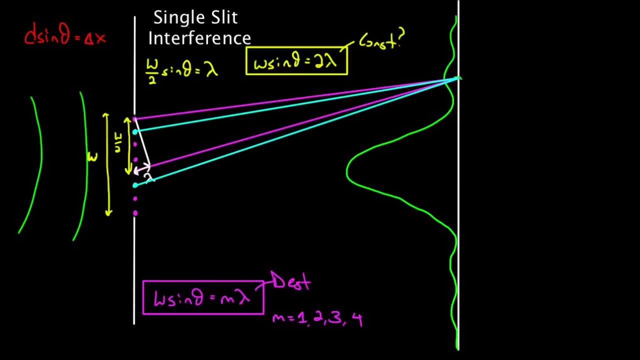 So far it's looking good. They're at the same angle, They're the same distance between them. I mean, this length here is still w over 2.. So I'd still get w over 2. Sine of the same angle because it's the same point on the wall. 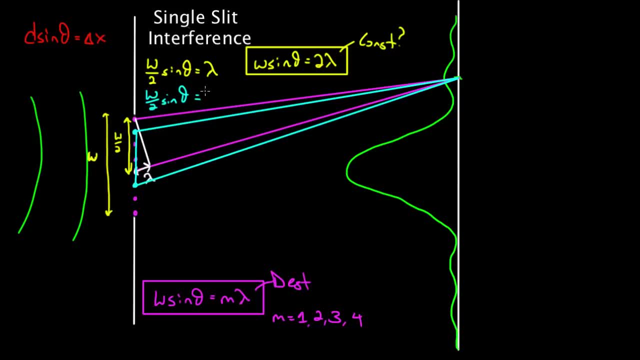 So if w over 2 is the same, sine of the theta is the same, then that's got to also be a path length difference of lambda, Which means these two blue waves also interfere constructively. So this is looking pretty good, which is kind of bad. 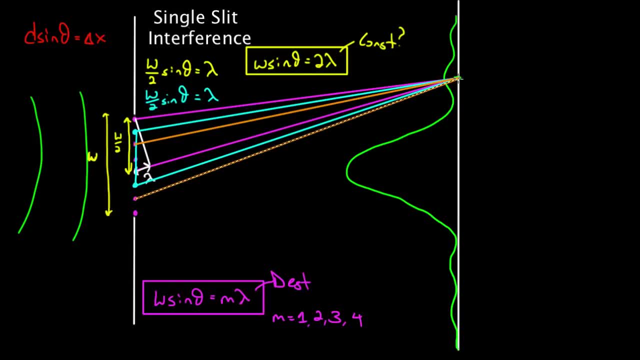 I'll show you why These two would also be constructive. Well, is this a constructive point? Is m equals to a constructive point or a destructive point? then? And it's a destructive point. This argument's failing. And it fails because watch this: 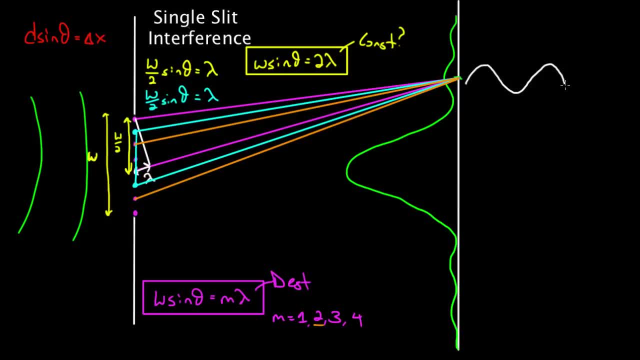 even though these two purple ones interfere constructively over here. here's a wave cycle, even though the two purple ones meet up constructively. let's say the top one was there, that means the one in the middle, this one here was also at the peak. 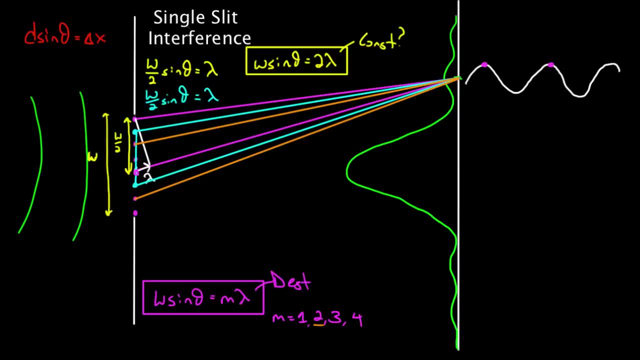 So those two interfere constructively. How about the next two? Well, those two are going to interfere. now, maybe those two are like at this point: They're both constructive, But they're not necessarily the same as the two purple ones. And how about the orange ones? 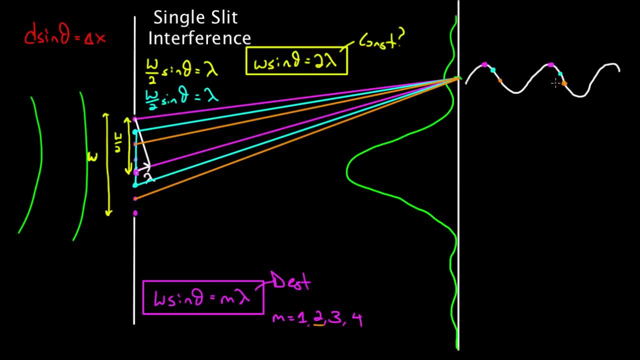 Orange ones might be constructive, because they're both at the same point in the phase, But they're not at the same point as all the rest of them. You can have more. What about these down here? Well, these might be down here. 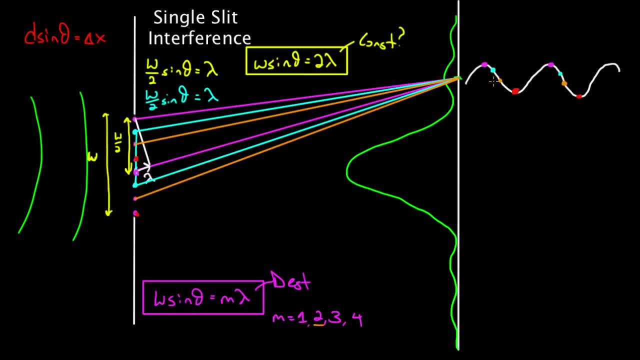 Those two together are also constructive. but you see the problem, Even though these two are constructive, this one's not constructive with this guy and these all add up, In fact, for the most part, they cancel. That's why these are so little. 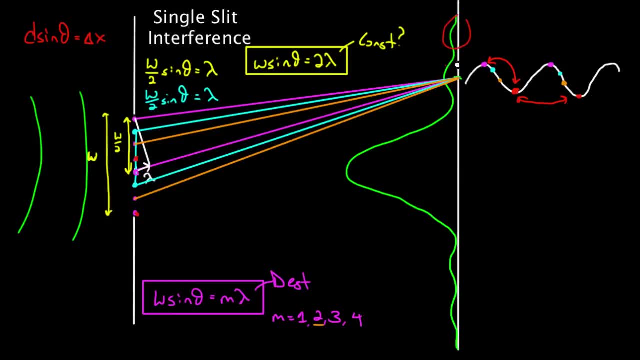 You get these weak. you get these really weak fringes on the sides of a single slit because you're not going to get points where they all add up really well. necessarily, You get points where a lot of them sort of cancel out. 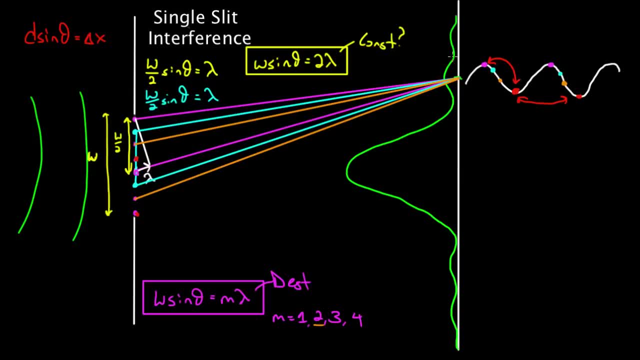 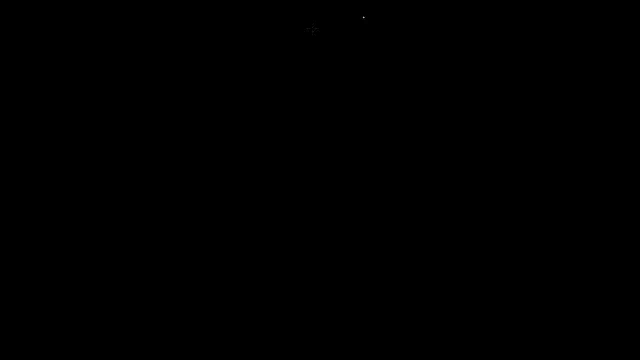 And it doesn't completely cancel, though Here's where I lied for the diffraction grating. Remember, for the diffraction grating. let me get rid of this. For the diffraction grating, we had a single line and we made a ton of holes in it. 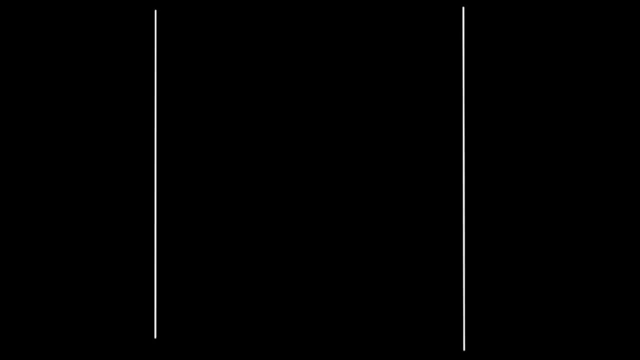 And I said that diffraction gratings are great, because if you come over here, you make a ton of holes in here. Instead of getting a smudgy pattern on the wall, you get a big bright spot right in the middle and then a well-defined, well-defined, well-defined. 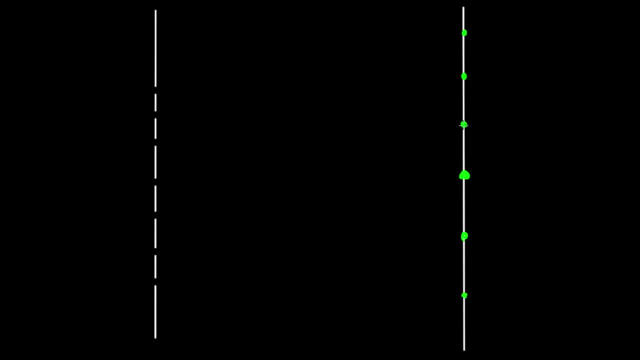 on each side of them evenly spaced. Basically just zero and then extremely sharp And then zero and then extremely sharp And then zero and then extremely sharp. And the whole argument I made for diffraction gratings was that the reason it's zero in between. 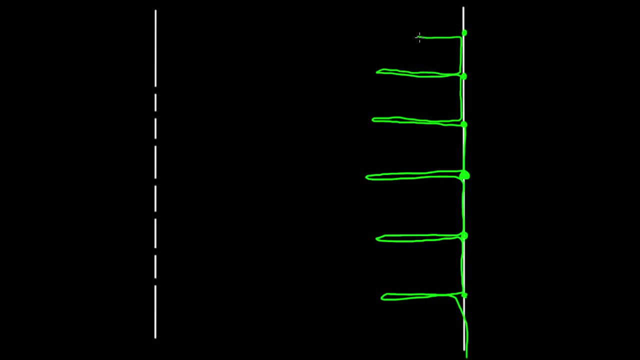 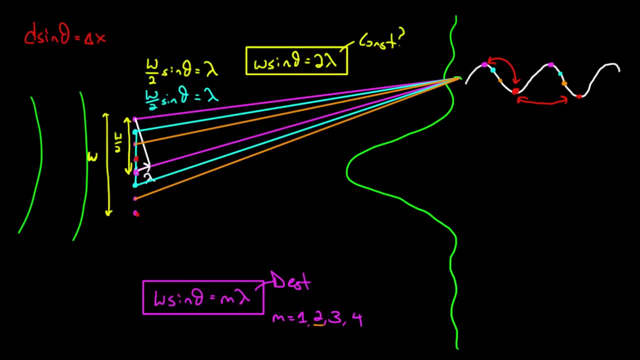 the reason these are giving zero everywhere except these constructive points, was precisely because, if we come back over to here, was precisely because of this effect right here, This effect where they, for the most part, cancel. Now I'm saying, eh, they don't actually completely cancel necessarily. 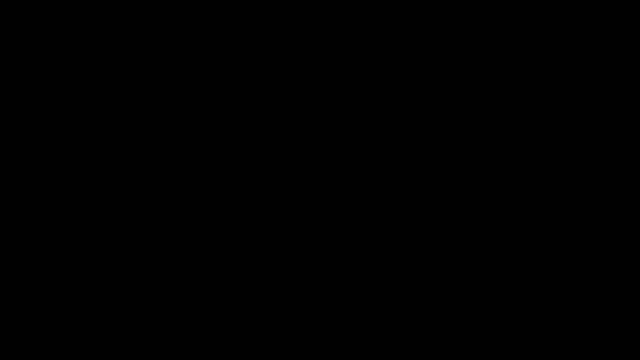 So these wiggles here are actually in a diffraction grating pattern. they're just so small and unpronounced compared to these you don't really notice them. What I'm saying is, if I wanted to draw this more realistically, 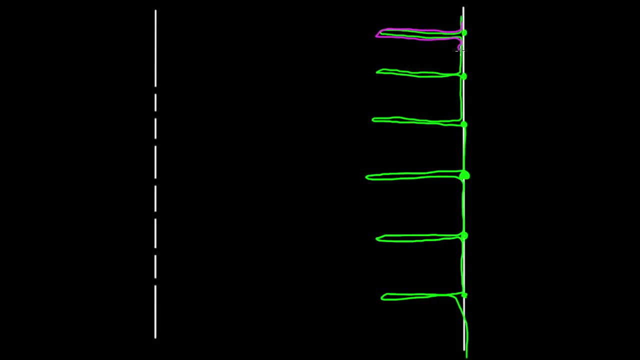 I would definitely have this bright spot right here, but I'd have this in between Small variations, Small points, where it becomes a little more or a little less constructive or destructive. What you have for a single slit is this, Just one center bright spot. 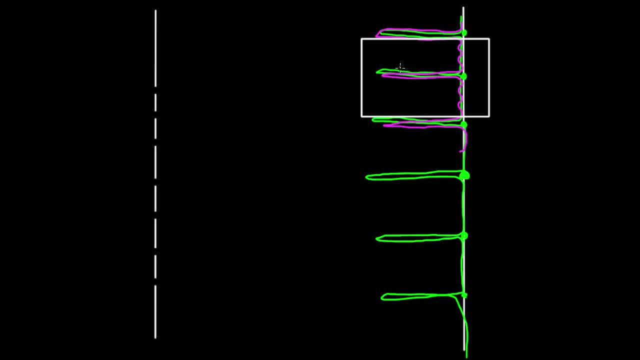 It's not going to be as well defined because it's not a diffraction grating, it's a single slit, But you still get these. You get these weird wiggles that for the most part, you ignore for a diffraction grating. 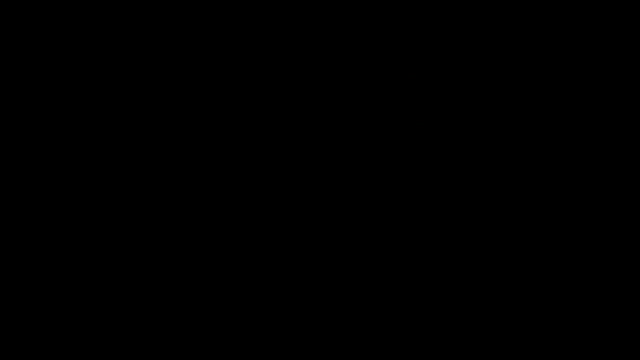 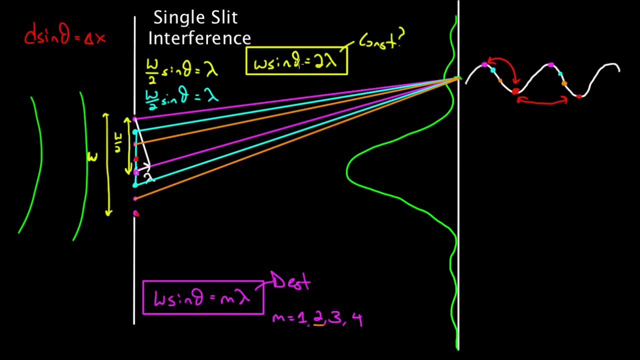 But they're there And for a single slit that's kind of all you got. So can't really ignore it so much. Those are going to be there. It's because these don't completely cancel, Our argument does not work. 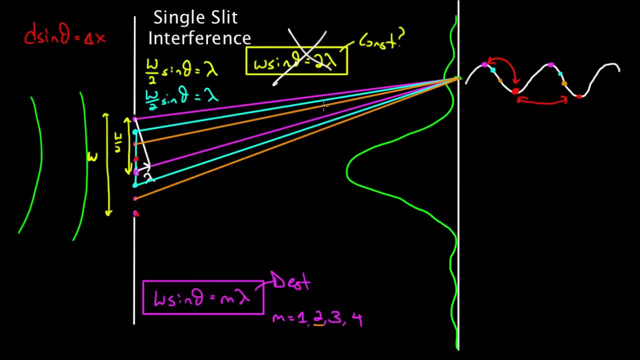 It works in the sense that two of these might be constructive. That means you can pair these off in constructive, but they won't all be at the same point on their phase, which would give you a completely constructive point there. So that's why we don't. 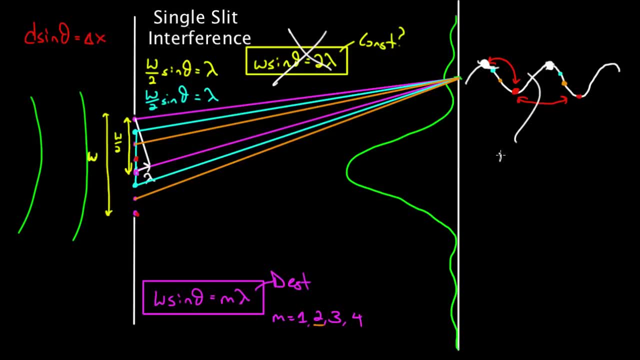 it's hard to find an exact formula. What's the formula for? For the constructive points? Well, getting this formula not quite as simple. You need to know a little bit more physics to do that, And so typically in introductory physics classes. 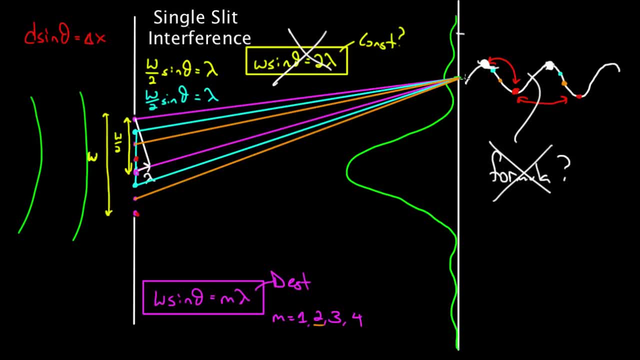 you aren't asked to find the exact locations of the most constructive points over here. Even these most constructive points partially cancel. You do know how to find the exact locations of the destructive points, though, And if you wanted an approximate location of a constructive point, 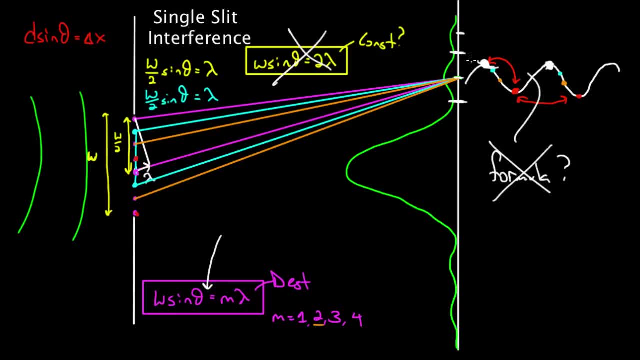 well, you can find the exact location of two neighboring destructive points, which, if you really wanted to, I mean the constructives in there- approximately in the middle, if you wanted to get a rough idea. I can still see some of you being upset, though. 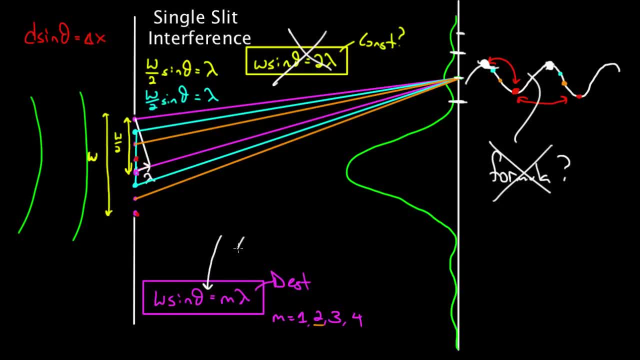 You might say wait, hold on a minute. So we're saying this formula's good for the destructive points, but is this problem we ran into for constructive points also a problem for destructive points? And it's not. It doesn't matter if they're at different points. 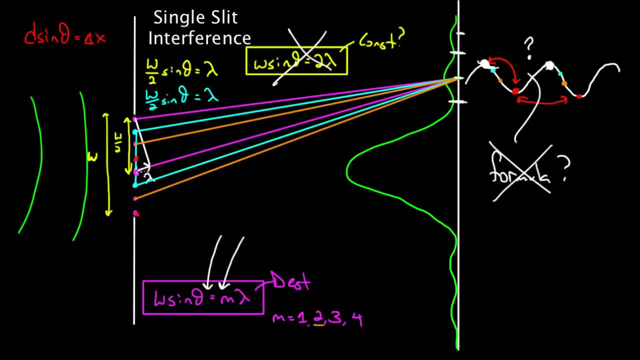 in their phase for the destructive, because each pair cancels. In other words, when we ran through this argument for the destructive points, lookit, if these two purple ones cancel, then they cancel. I mean, if one was at the peak. 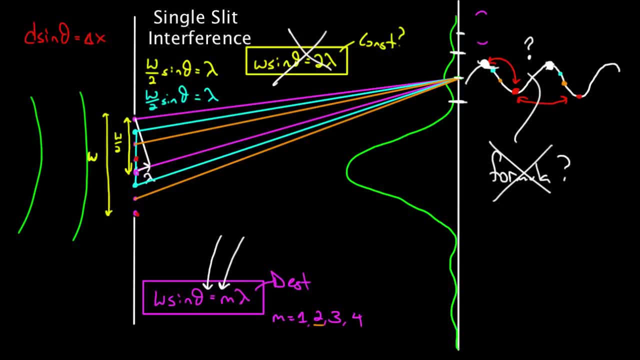 and then the other's at the trough or the valley. those add up to zero. They're gone. Any effect they might have had on light hitting this point in time when the screen is gone, completely negated. And so what about the next two? 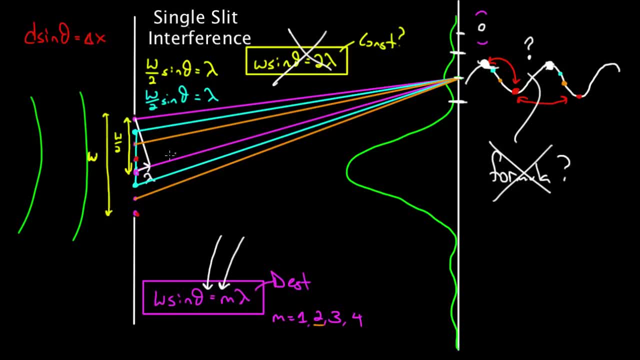 These two blue ones? Well, those two. if these two purple ones cancel, remember, the argument went that these two blue ones would have to cancel. So no matter where they're at, they're at some different point on the cycle. Let's say one's here and the other's. 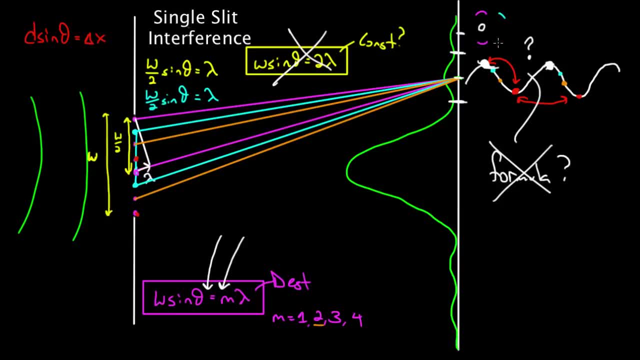 well, that looked like the same. So let's say one's here and the other's at this corresponding 180 degree out of phase point. Well, they still cancel. That adds up to zero, And so it doesn't even matter. 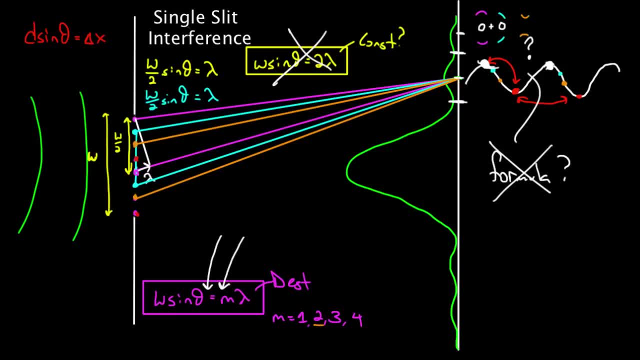 that they're at different points in their phase, It doesn't matter. no matter where they're at one's 180 degrees out of phase with the other, Every contribution cancels out. You add up a bunch of zeros, you get zero. 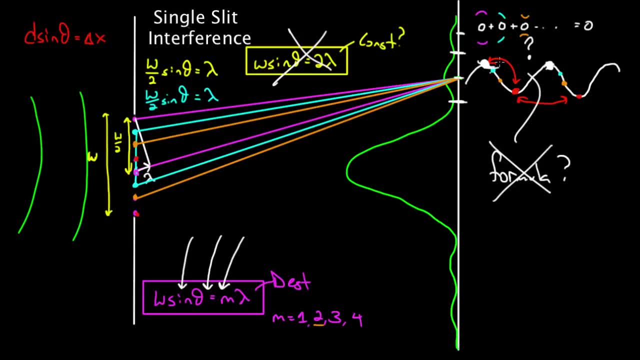 So destructive works fine, You don't run into the same problem with constructive. It's a problem for the constructive points because these might add up to some big number and then the blue ones add up to a different number and the orange one adds up to a different number. 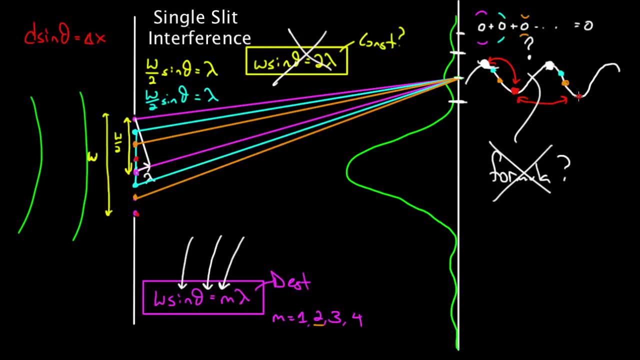 and then the red ones might add up to a negative number. and you keep getting these different numbers. You try to add them all up. Well, what do you get? That's why this formula's not so easy to find. Adding up zeros, that's easy. 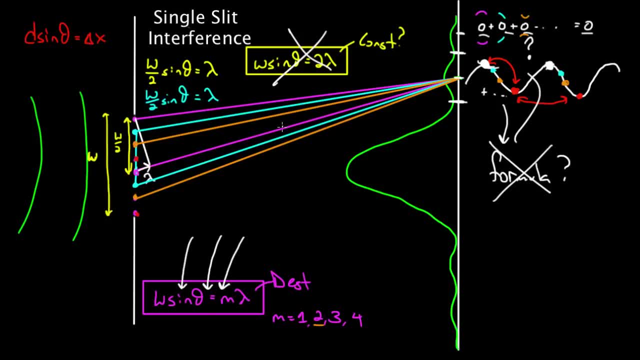 It just gives you zero. So I hope I showed you that this crazy mumbo jumbo argument can't say anything whatsoever And hopefully that gives you a little more justification. Hopefully it makes you believe a little more into this formula that we derived. 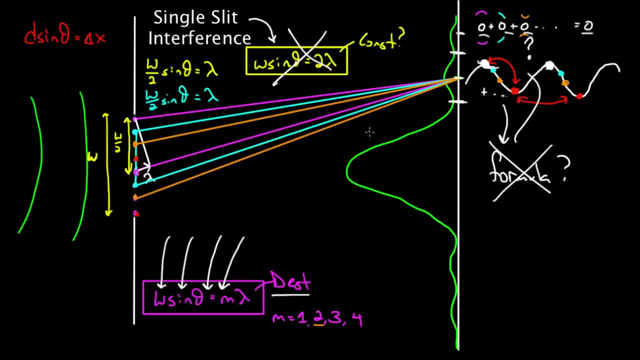 for the destructive points, Those it does work for, And so we can find destructive points, just fine. One more thing we can find is the width of this center bright fringe. here, the center bright spot, It's going to be wide, And since this goes to m equals 1,.